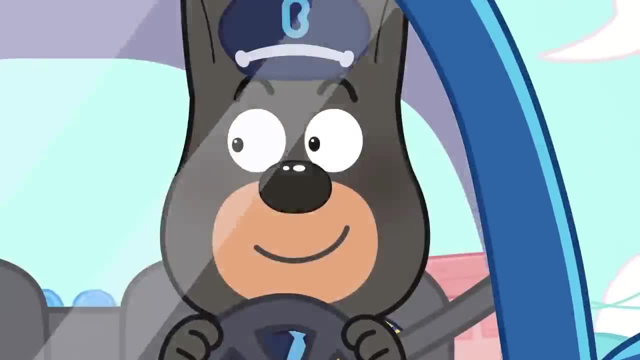 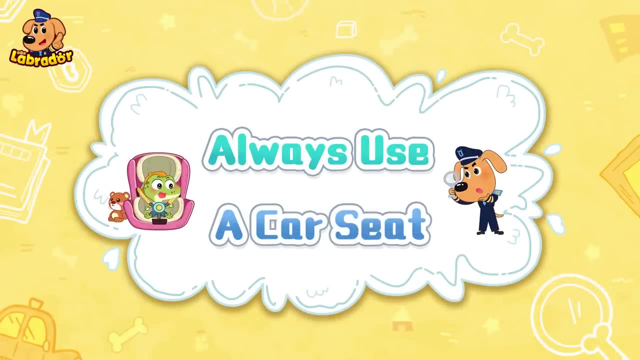 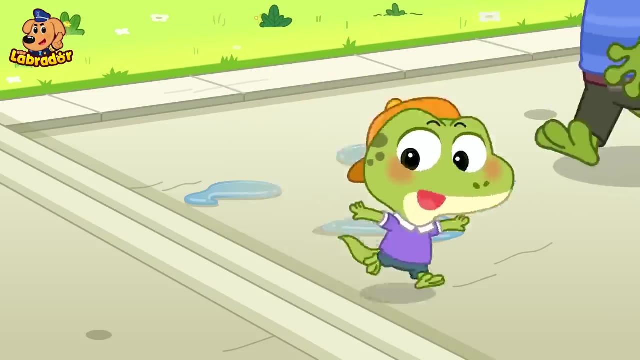 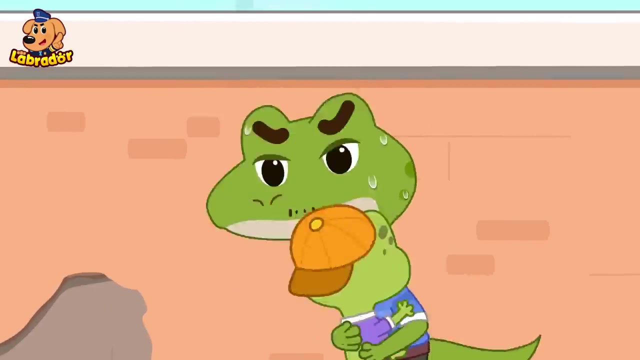 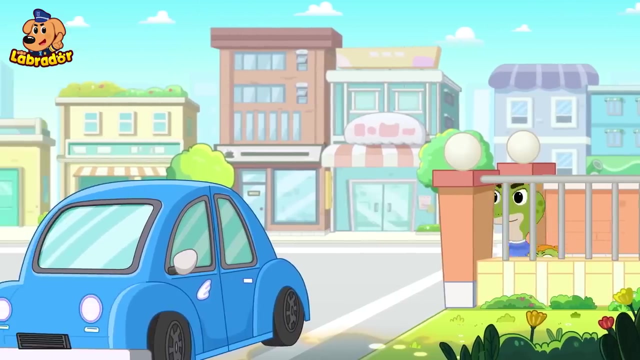 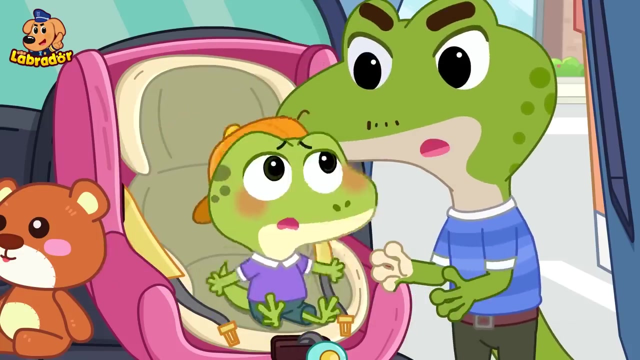 Go, go, go go. Let's go. Sherry Labrador, Always use a car seat. I'm going to the amusement park. Sweetie, don't climb up high. You should walk carefully. Oh Daddy, I don't want to sit in the car seat. 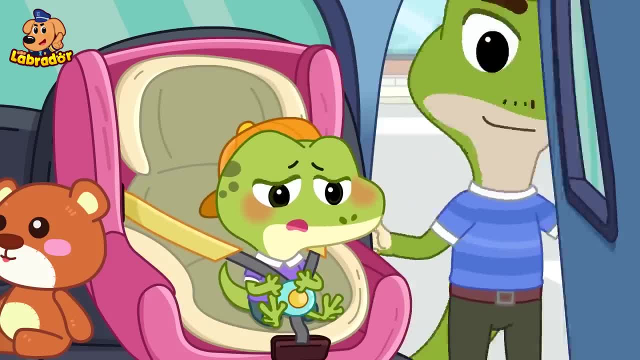 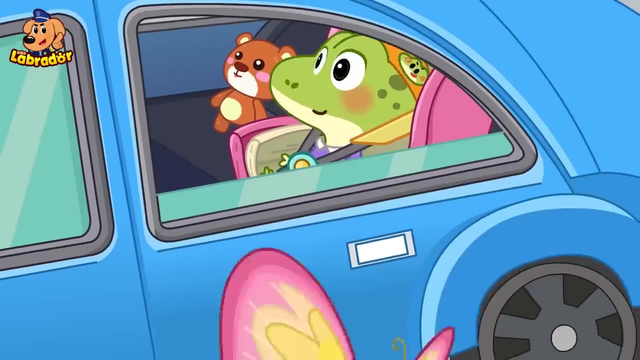 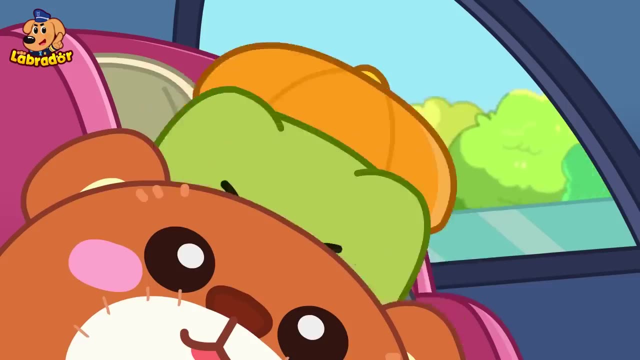 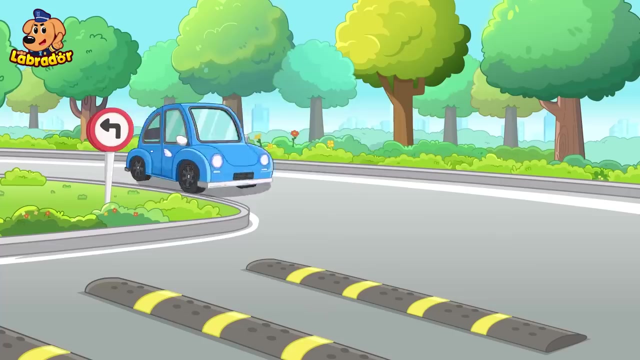 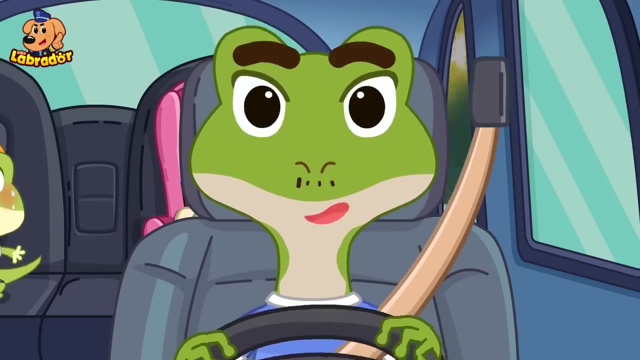 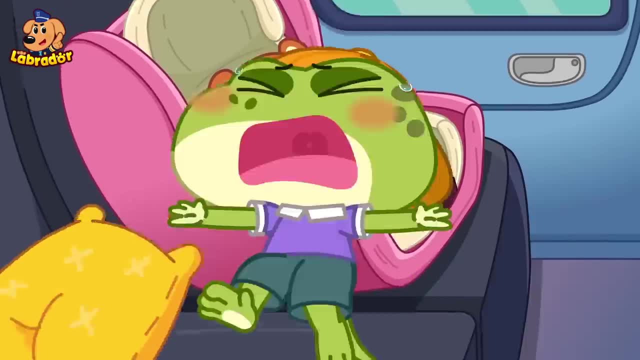 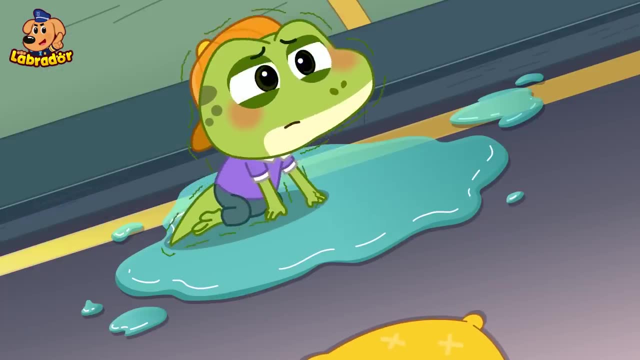 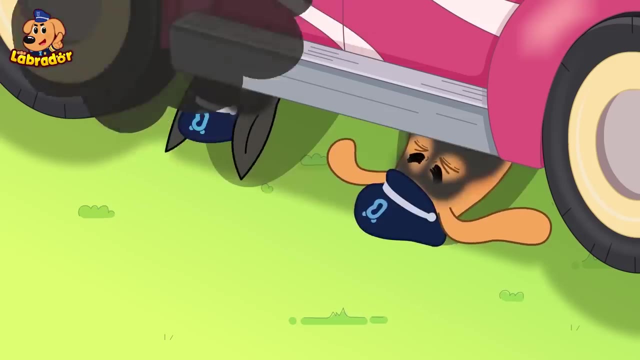 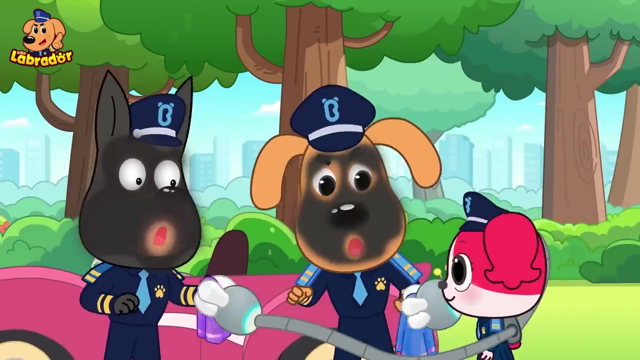 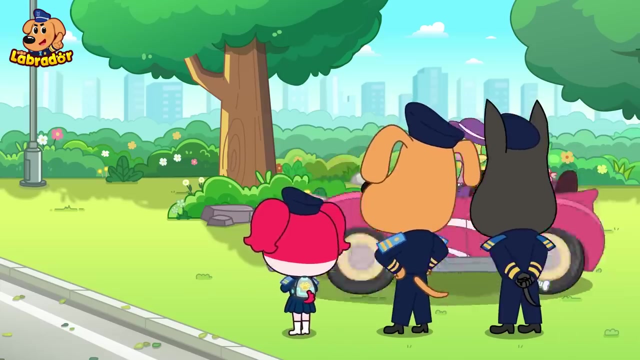 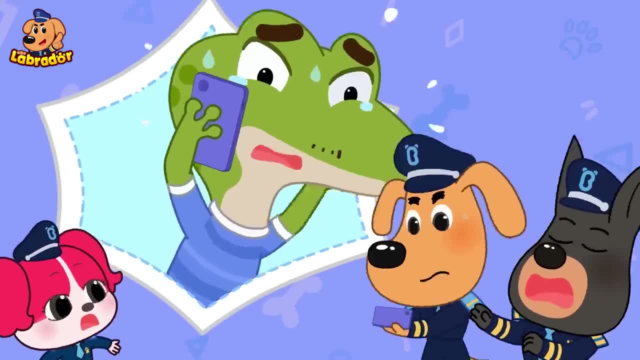 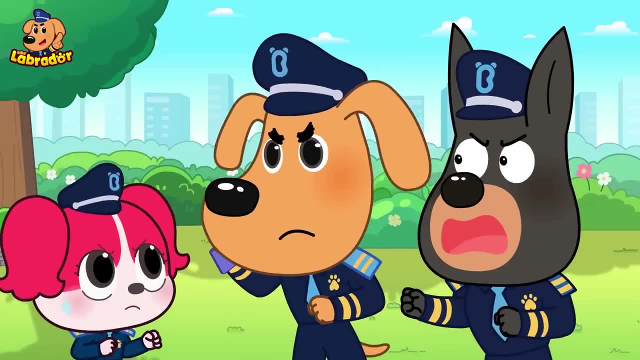 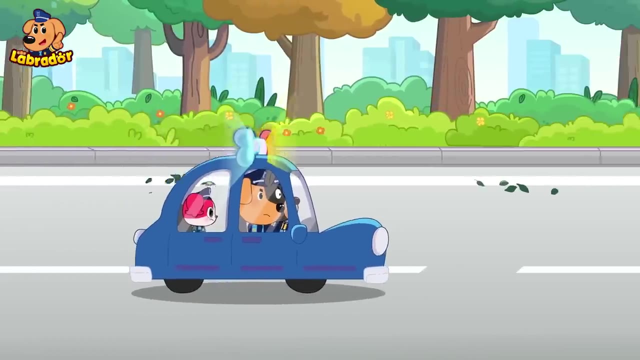 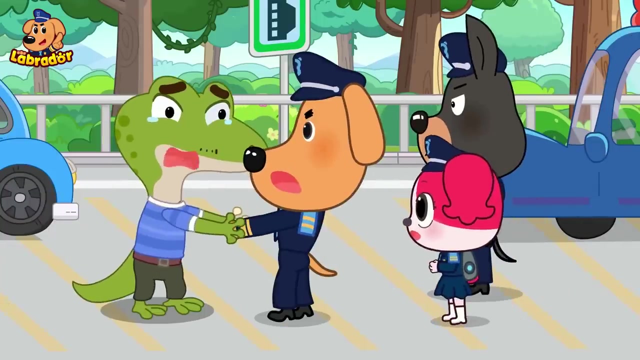 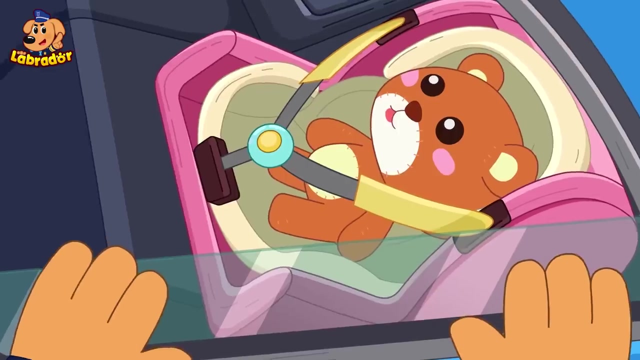 Hi, I'm Sheriff Labrador. Sheriff Labrador, My son was just in the car and suddenly disappeared. Please help, We'll be right there, Sheriff Labrador, Don't worry, Let us check first. Ah, looks like he wasn't sitting in his car seat. 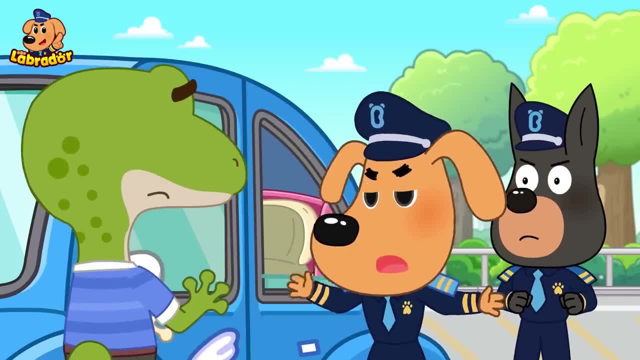 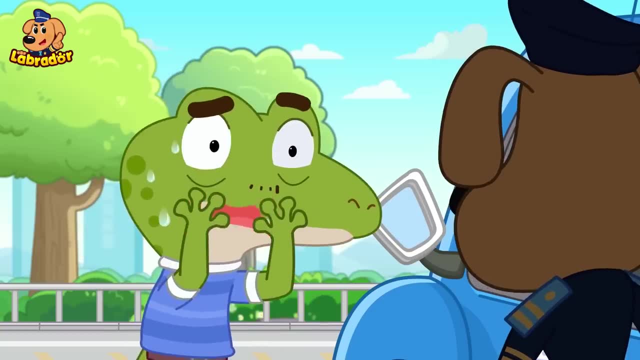 Mr Gecko, did anything unusual happen while you were driving? Yes, A piece of newspaper blocked my view, so I had to make a sharp turn. It seems like little Gecko was thrown out of the car because he wasn't sitting in his car seat. 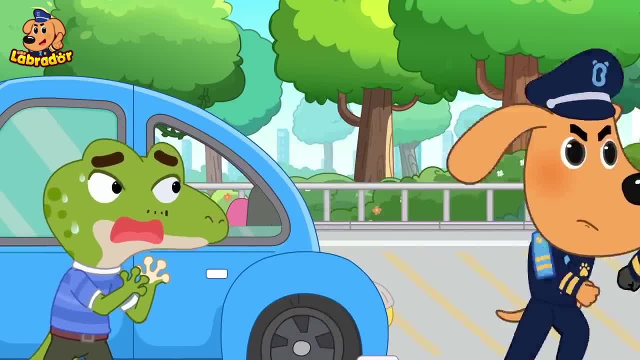 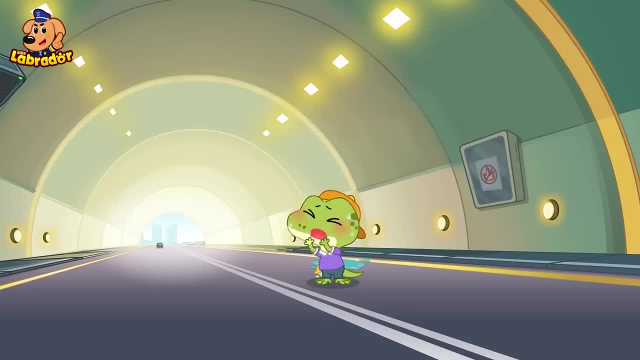 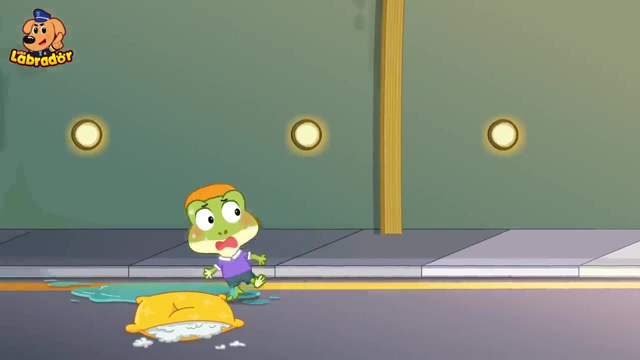 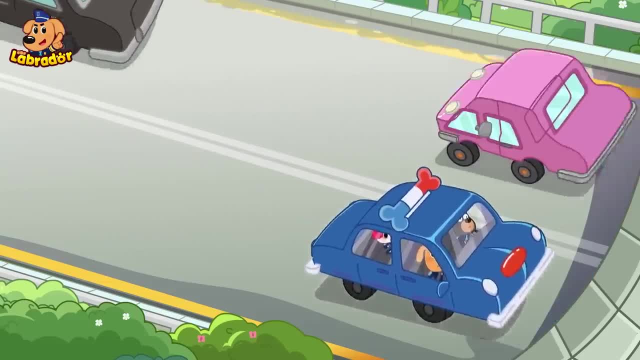 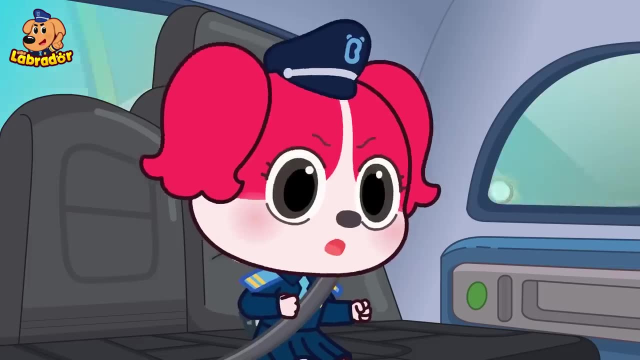 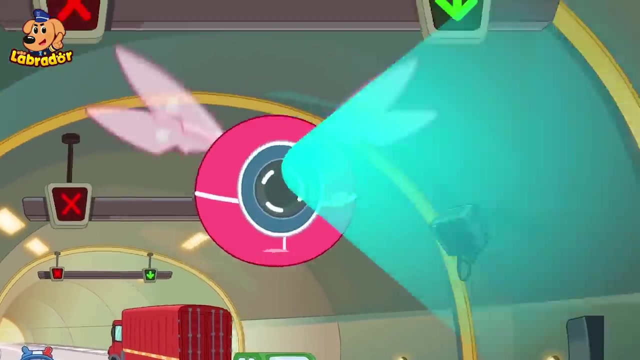 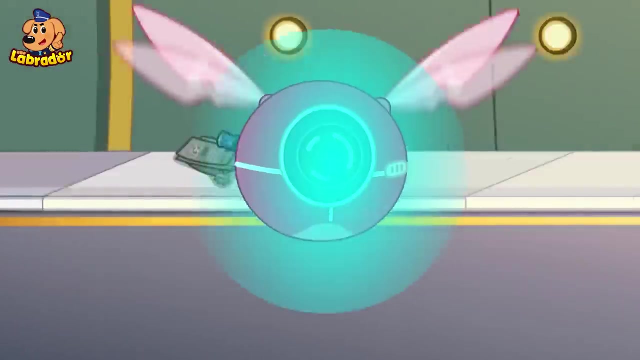 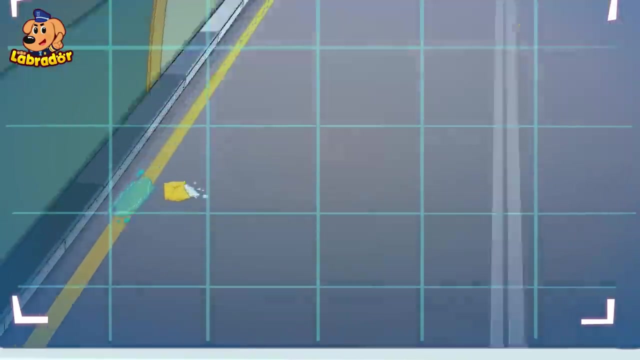 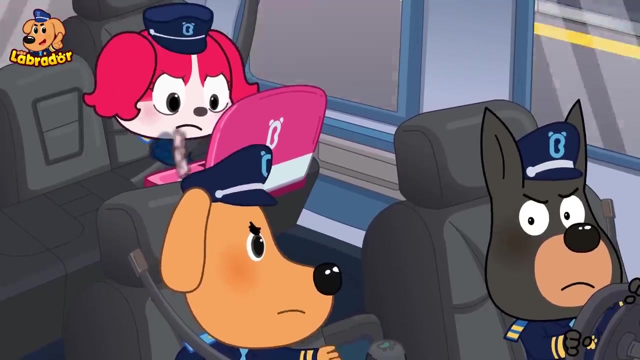 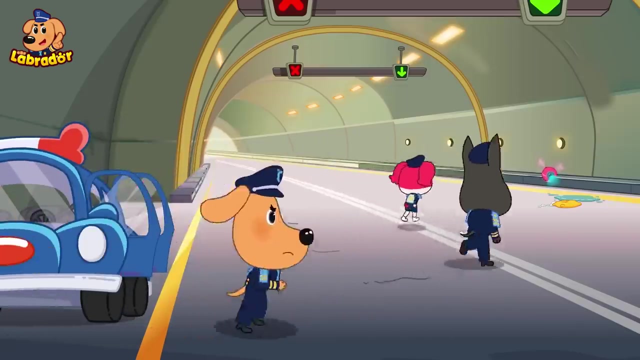 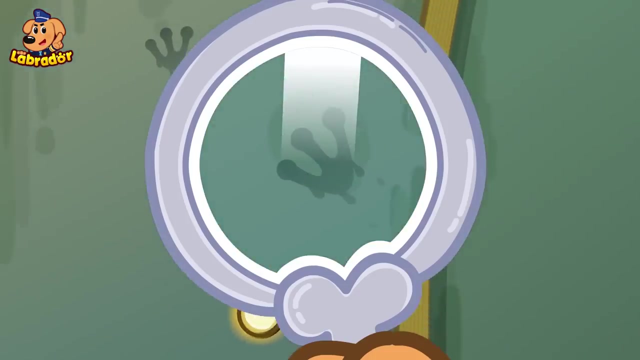 Daddy, where are you? Papillon search with your super flying eye. Got it. Little Gecko, where are you? I found a cushion on the ground. ahead, Let's go. I think this is Little Gecko's cushion, Ah, And these are his footprints. 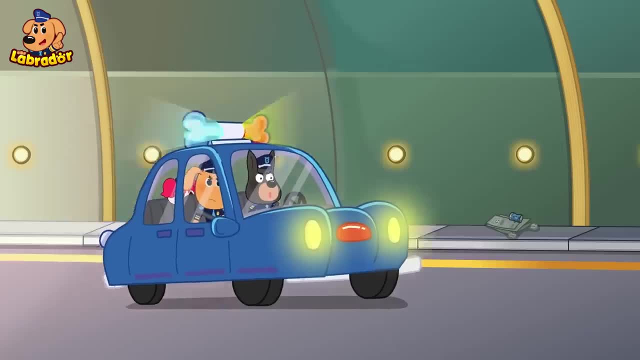 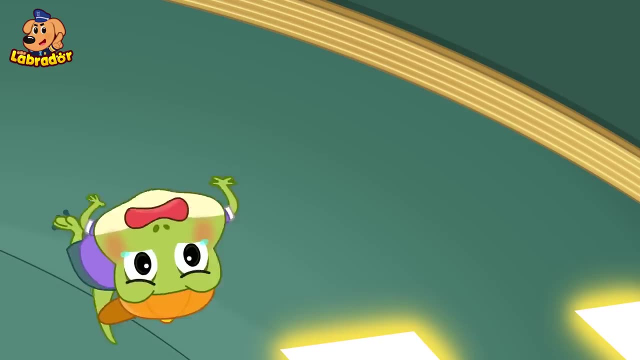 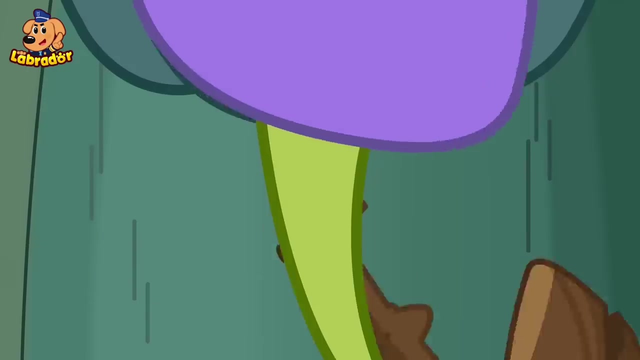 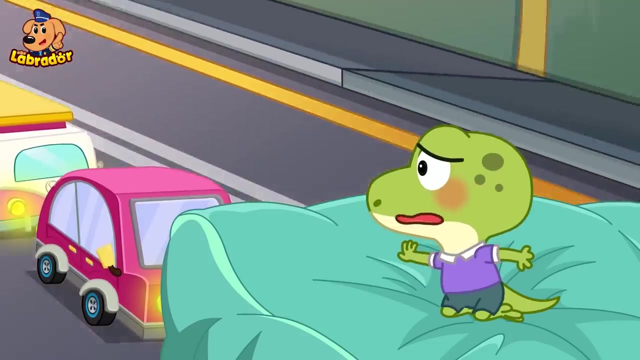 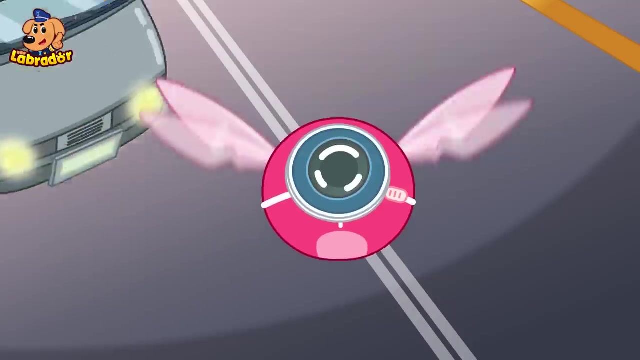 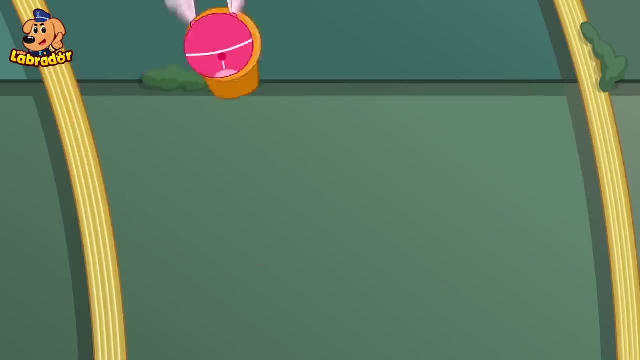 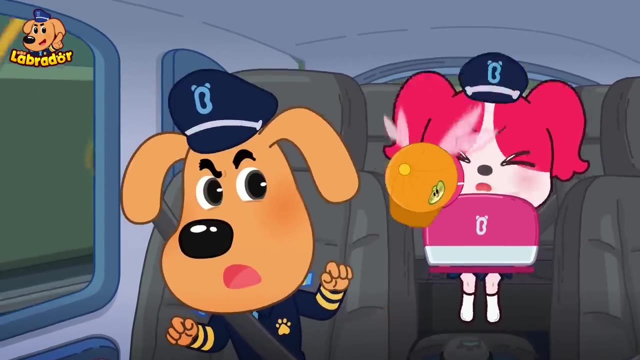 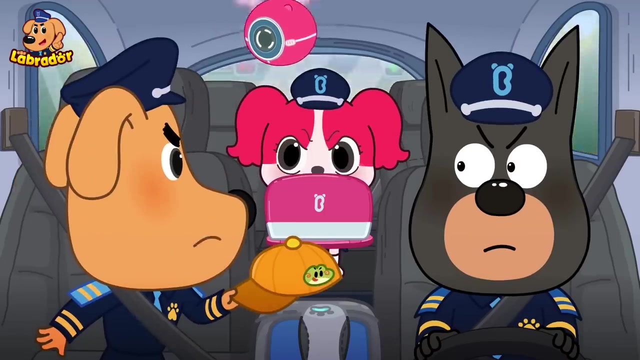 Huh, What's that Error? Error Returning. now It's Little Gecko's hat. Oh no, He might have fallen. He might have fallen on that fan ahead. Hurry Doby, Leave it to me Ha.